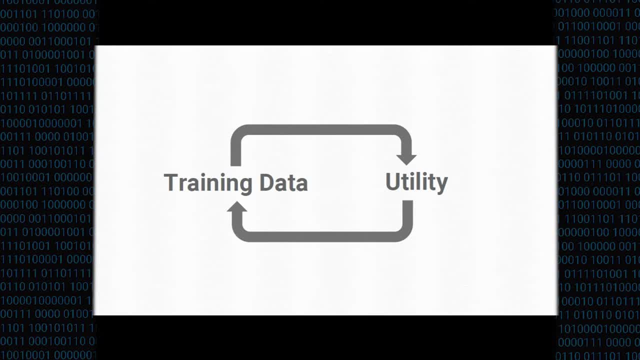 by increased by high utility of applications, share more and more data with their devices and computing platforms, Who in turn become more powerful and useful to end consumers, As the shared data is becoming more personalized and sensitive, it's upon us security researchers. 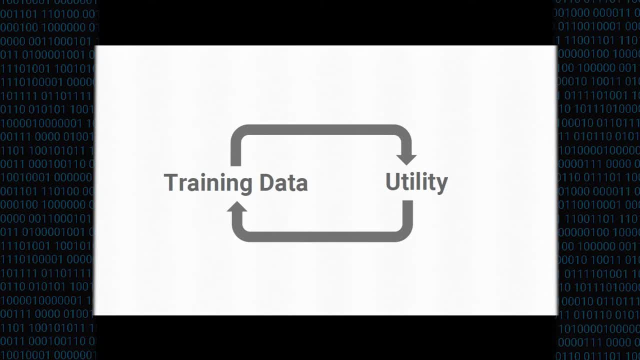 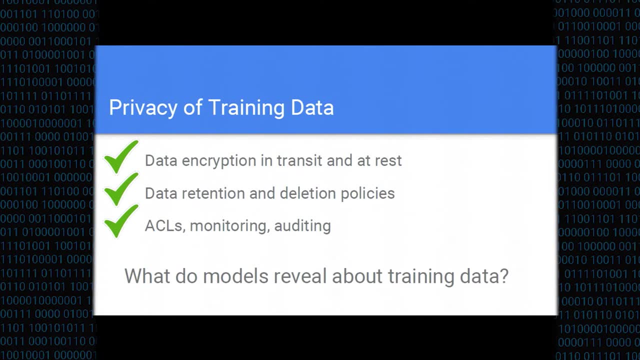 to give the training data protection it deserves And, of course, I take it for granted that we are going to apply and use industry's best practices in data encryption, data retention, access control and data security. Thank you, Thank you. 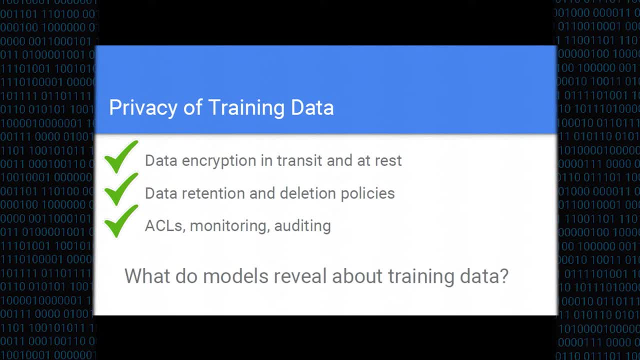 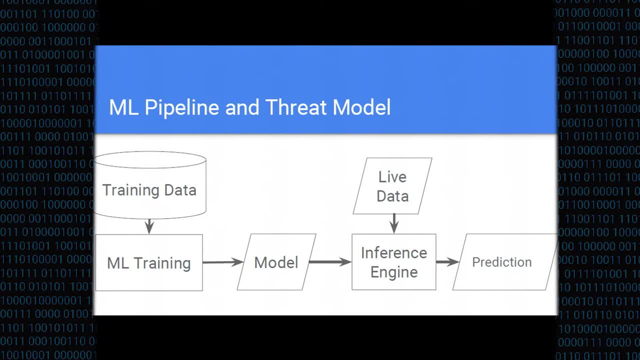 And this is a standard pipeline for a machine learning task, where training data is used to fit a model that is then used by inference engine to make predictions. Even though we might only care about privacy of the prediction, we don't care about privacy of the prediction. 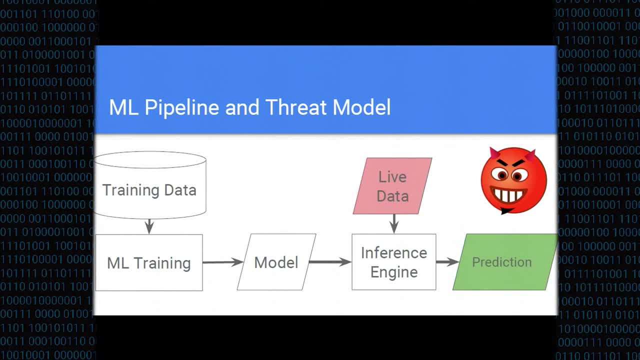 that users see An adversary is generally able to feed its own inputs into the inference engine. It may even get its hands on the model itself if it's shipped to end-user devices. So our best bet to protect privacy of training data is ensuring that the model itself is privacy preserving, And the focus of this. 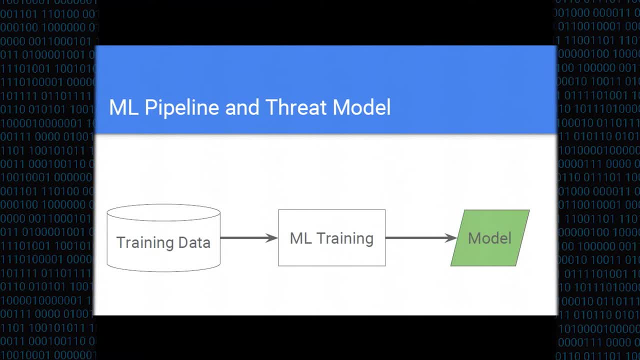 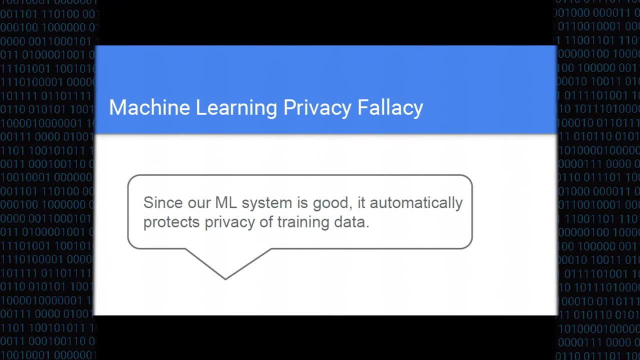 talk is going to be on this transformation of taking and training data and fitting a model that preserves its privacy, And here I would I want to call out what I term a privacy learning or machine learning privacy fallacy that you can hear from from machine learning researchers or data scientists who 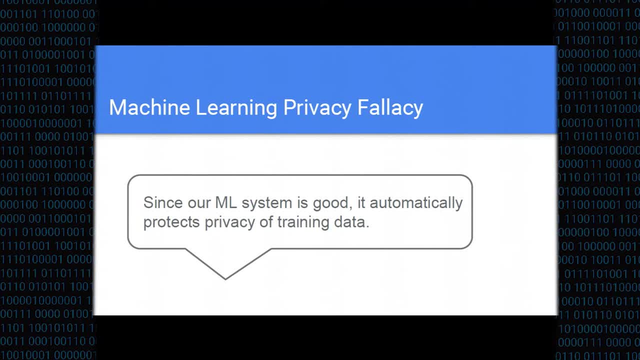 would say that a well-trained machine learning model would preserve privacy of underlying training data, because, well, it's good, it's trained on a massive amount of data. and I won't challenge this belief And these are reasons why I believe I think. 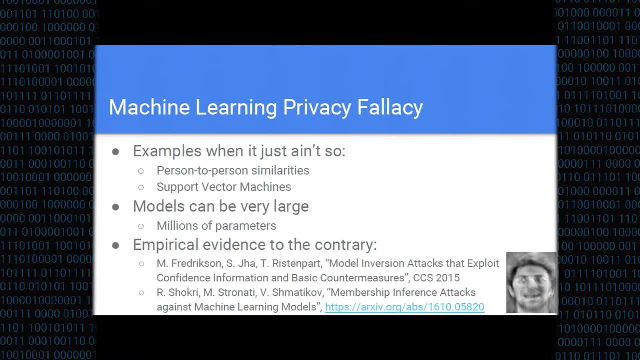 that this is actually wrong in many important cases. So, first of all, there are examples of good quality machine learning models that just fail to protect privacy. One example would be a recommender engine based on user-to-user similarities: If an adversary is able to come up with a. 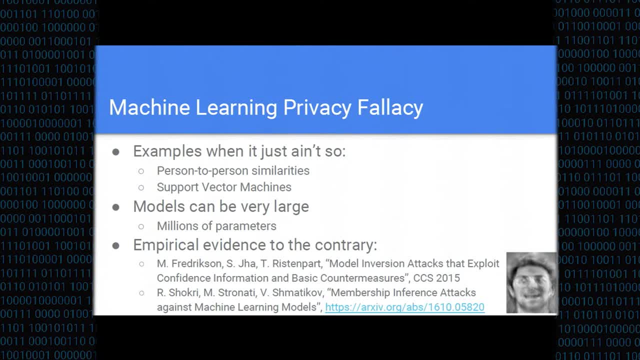 profile that comes sufficiently close to yours, the system will happily fill in the gaps if it is based on user-to-user similarities Support vector machines. It's a well-known machine learning technique that by design and explicitly includes as part of its model records from from the original data. 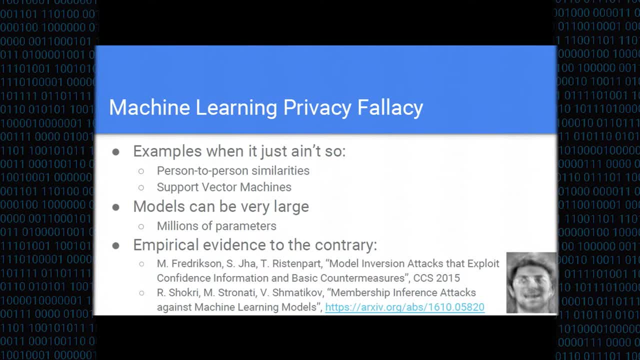 set, Then models can be very large, can be can include hundreds of thousands or even millions of high accuracy parameters, And I challenge anyone to argue that these models protect privacy of underlying data, and the burden of proof must be on people who make such claims. 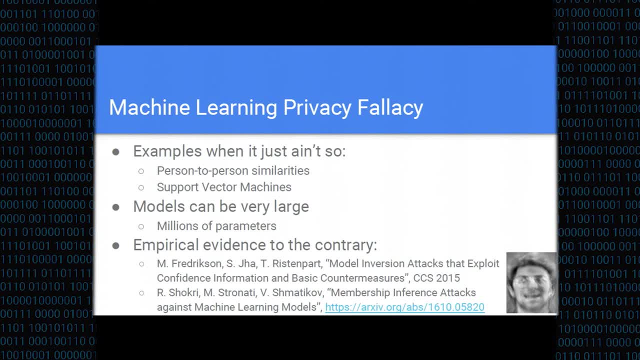 And there's also empirical evidence to the risks that are presented by machine learning models. There was a paper from last year's CCS that demonstrated that extracted images from a face recognition system that look suspicious like images from the underlying training data set. There's a very recent work by Shokri and others out of Cornell Tech that demonstrated 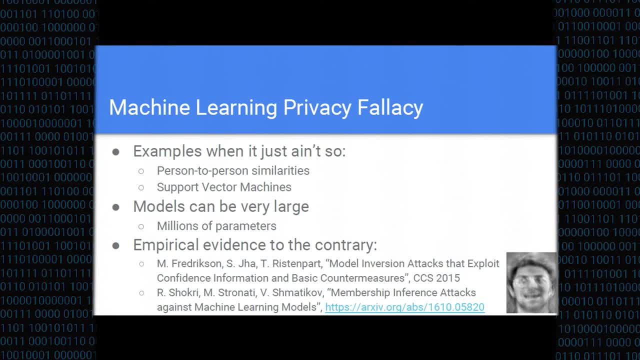 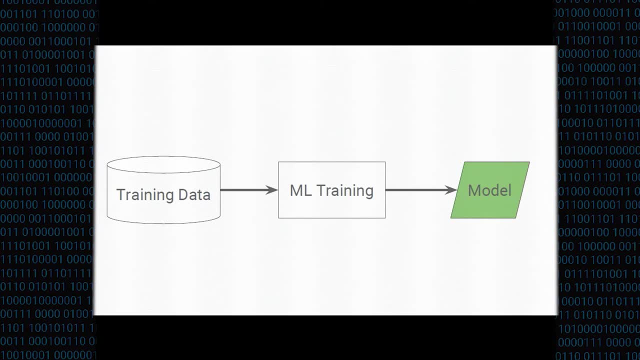 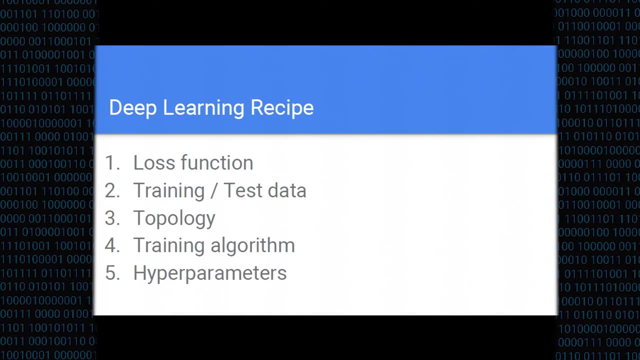 a powerful membership attack on the machine learning system. So Before we think about ways of doing machine learning with privacy, let's understand how it's done with out privacy. So this is a very rough recipe for the pipeline for deep learning training. So we have to pick a loss function, the function we want to optimize. We take account of data and 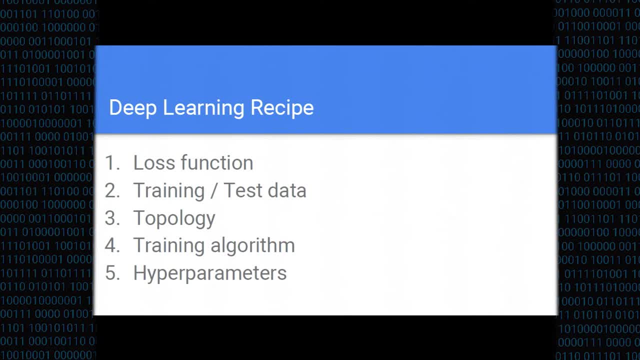 load it in an emotional sigh. Ah, if we use a ludicrous Pour I spread, we have to pick a loss function, The function that we want to optimize. We take account of data, of available training and test data sets. We choose a topology of the network. 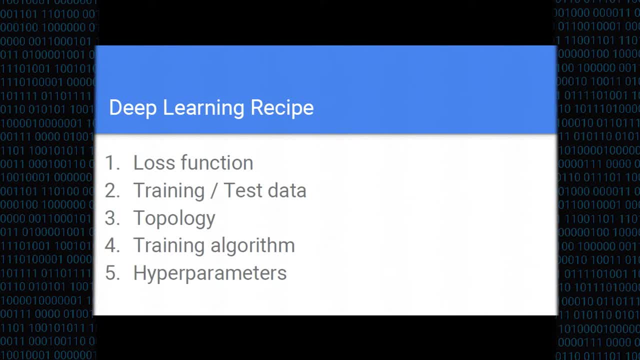 We select the training algorithm And we decide on hyperparameters such as the stopping rule or the learning rate, And we run it to completion. In this work, we'll be using softmax loss, which is a differentiable proxy for the accuracy of the classifiers we want to train. 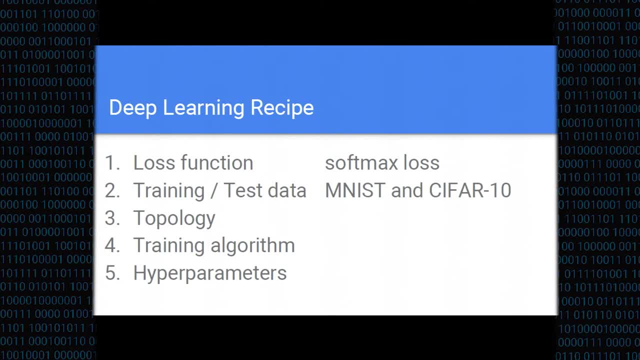 The training and test data sets are going to be two standard data sets used in machine learning, which I'll introduce in a few slides, But it's important to note that the yardstick by which we measure our progress is existed prior to our work. 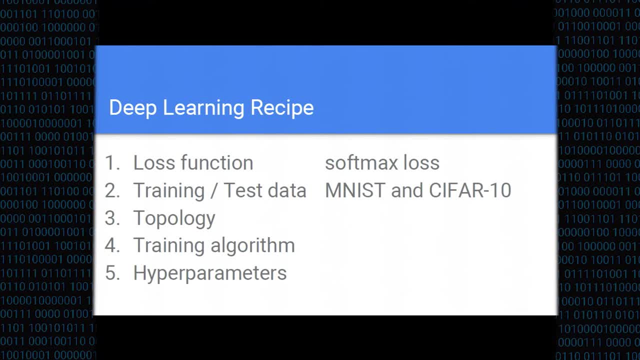 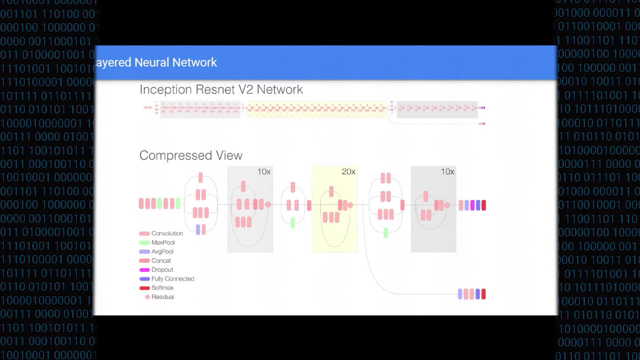 So we keep ourselves honest by comparing ourselves to existing, to prior art, For the topology of the network. we'll be using layered neural networks And this is an example of one. We'll be using a fairly deep neural network. We'll be using a much shallower network. that 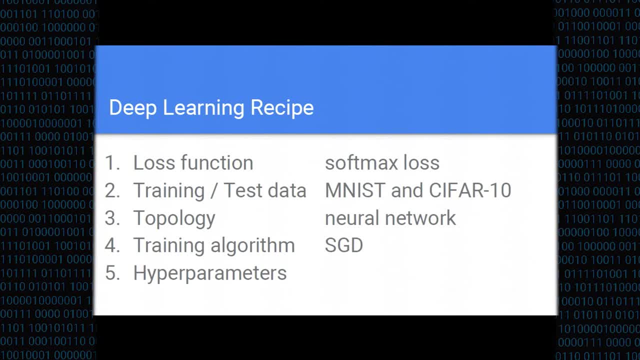 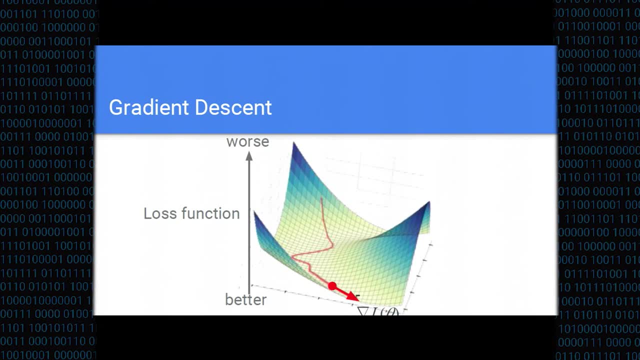 consists of just a few layers. The training algorithm is going to be stochastic gradient descent, which I'll explain over the next few slides. So the plane gradient descent minimizes a loss function by starting somewhere on the parameter plane and then updating the parameters in the direction where the loss 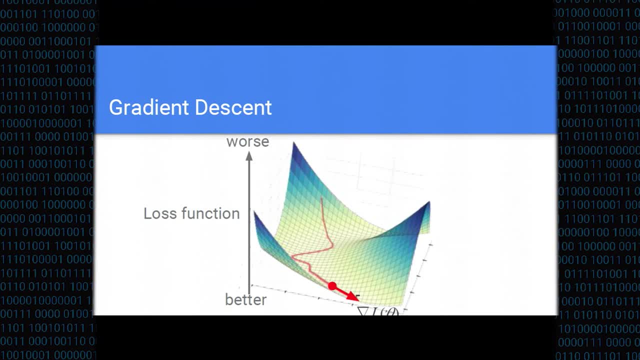 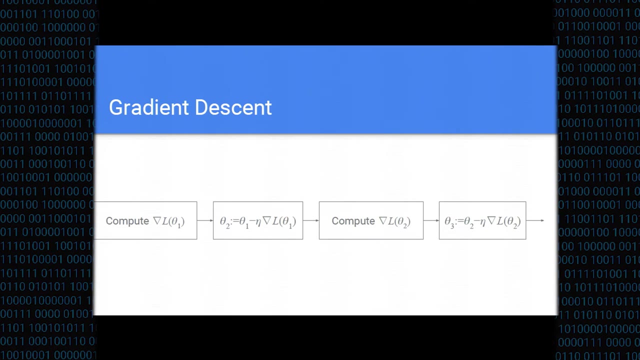 function decreases the steepest Algorithmically. it consists of computing the gradient of the function, making a step in the direction opposite of the gradient, and do it again. Computing the gradient of the loss function can be a rather expensive reposition because it requires visiting every work. 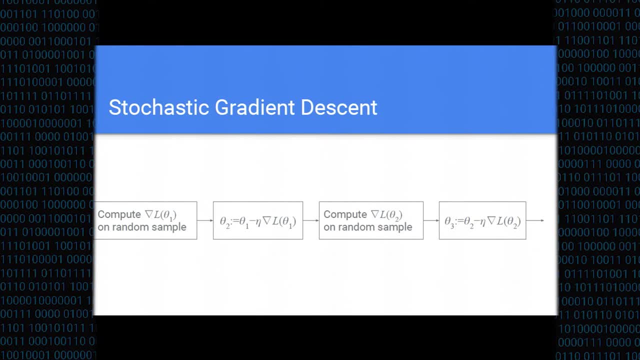 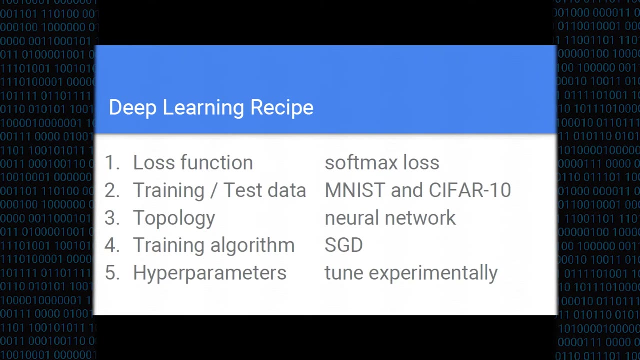 into the training data set. So instead we'll be running a stochastic gradient descent. This is an approximation to the loss function, which approximates it on the small sample of the training data. So this is the recipe for deep learning And, as you can imagine, there's no surprise here. 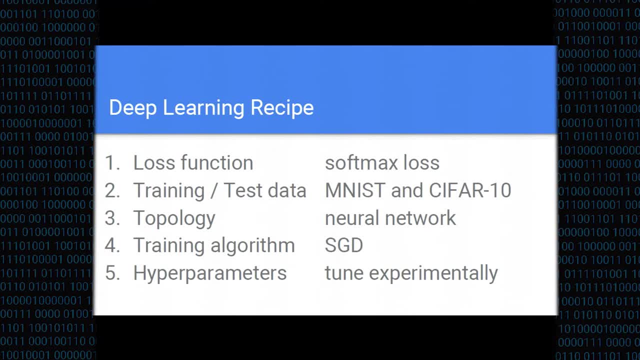 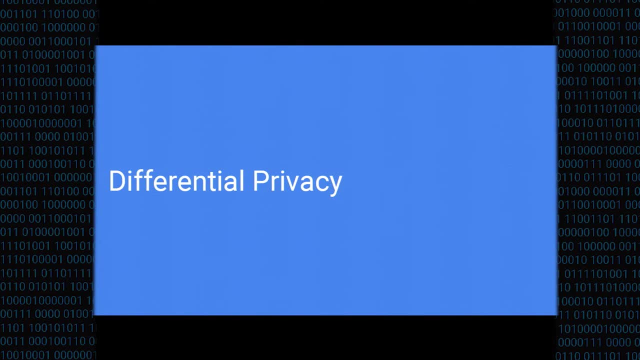 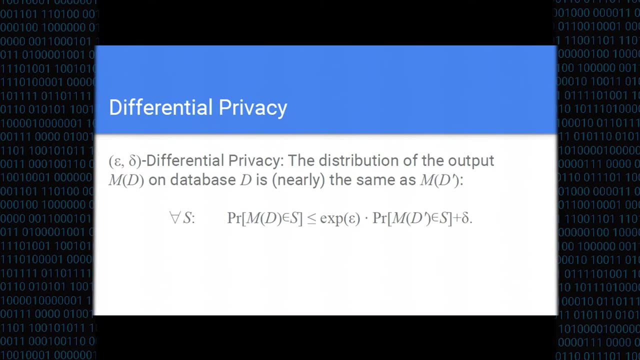 Our best bet of endowing this with privacy is by OK, so I hope that, yeah, But is endowing this with is to use differential privacy? In this work, we'll be using the epsilon delta formulation of differential privacy that states roughly: 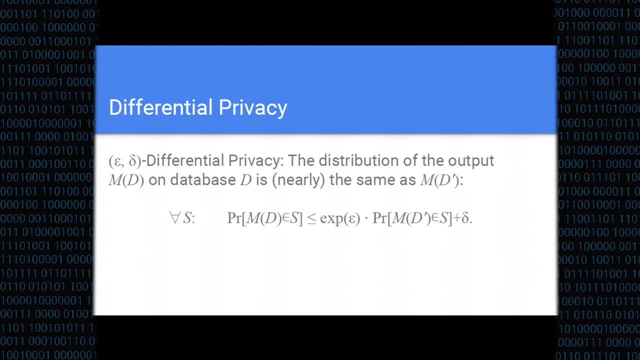 that the mechanisms of output on a database D is going to be nearly the same as the distribution of the output of the same mechanism on the database D prime, where D and D prime differ. And this definition has two parameters, epsilon and delta, where epsilon quantifies information leakage. 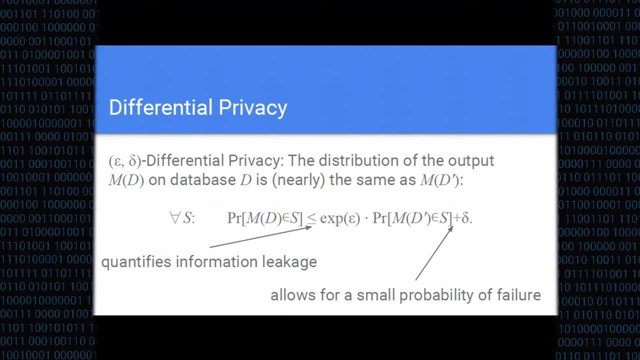 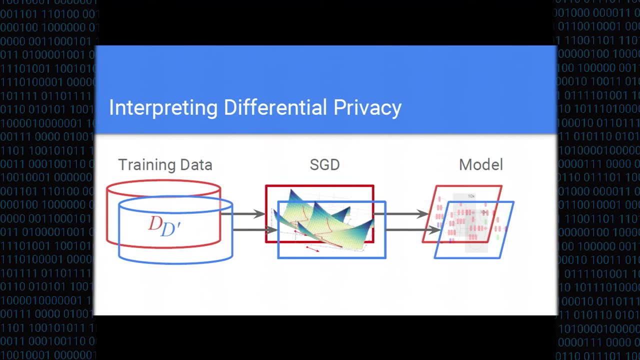 and delta allows for a small probability of failure. In the language of our machine learning example, differential privacy states that an adversary who examines output of the model trained on two different data sets- D and D prime- can't tell whether the model came from the blue distribution trained on D or sorry. 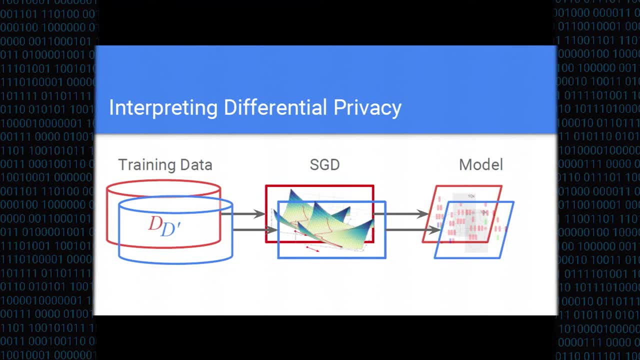 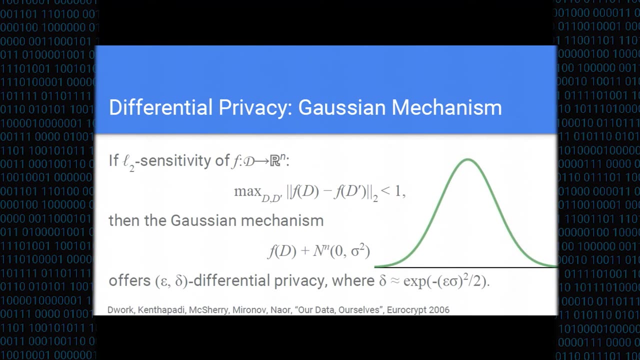 from the red distribution trained on D, versus the blue distribution where the model came from, the mechanism run on D prime. An important mechanism that we'll be relying on is going to be the Gaussian mechanism that approximately approximates an arbitrary function with a real-world output. 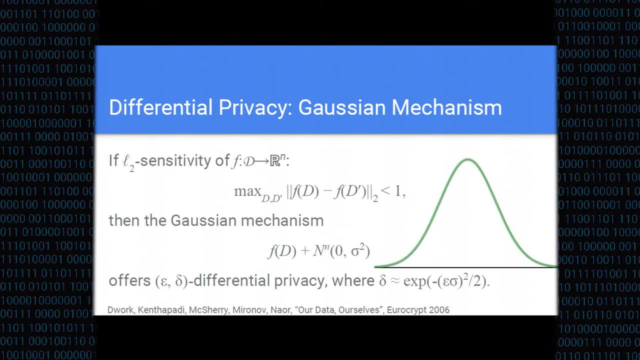 or a multidimensional output by adding a noise sample from the normal distribution where the parameter of the noise is calibrated, selected on the basis of the function's L2 sensitivity, which is defined as the maximal distance of the function's output, And it's the L2 norm. 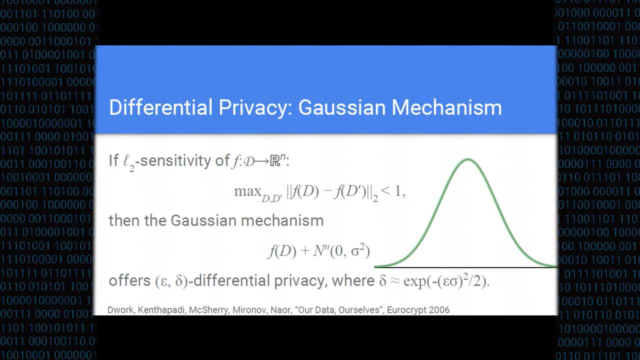 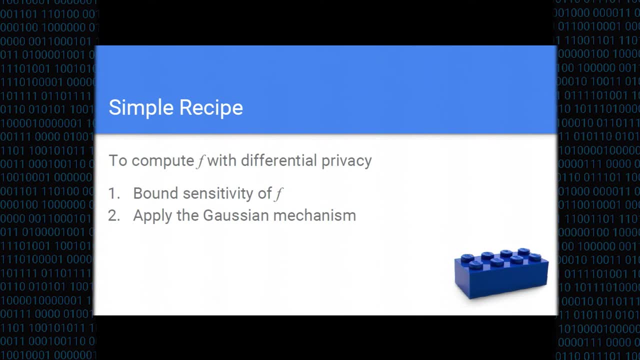 So we can see that the function is not using a very high-end function. It's using a very high-end function. So let's look at a simple example. This is a very simple recipe for computing a function with differential privacy. Step one: bound the sensitivity of the function. 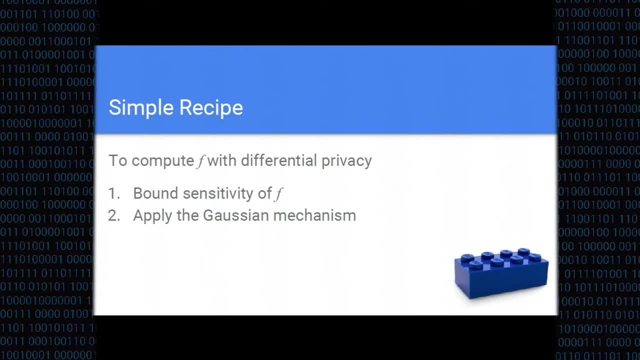 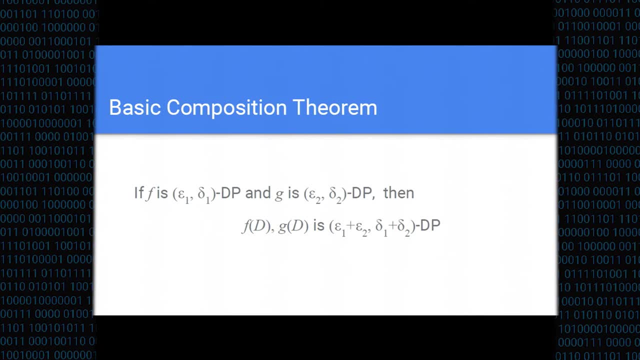 Step two apply a Gaussian additive noise mechanism. But what about functions whose sensitivity we cannot really analyze? Here a very useful property of differential privacy comes in useful, which the property is that differential privacy is composable and additive If two functions- f and d- are separately. 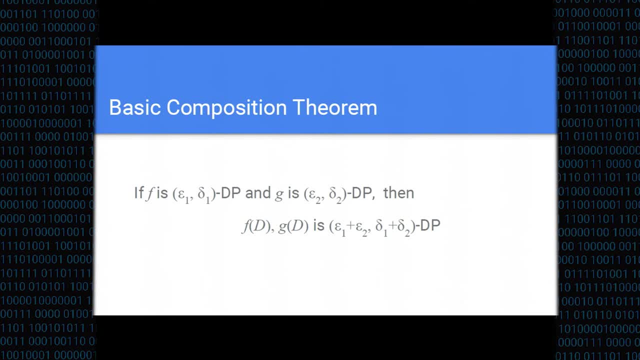 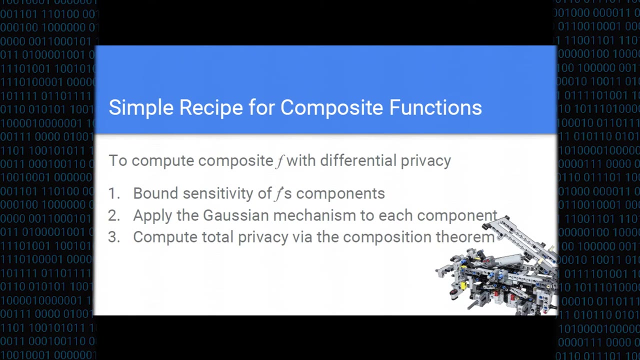 differential private, then releasing the output of these functions on the same input will be differential, private and the privacy parameters will add up. So it's just a recipe for computing a composite function with differential privacy that consists of bounding sensitivity of the function's components. 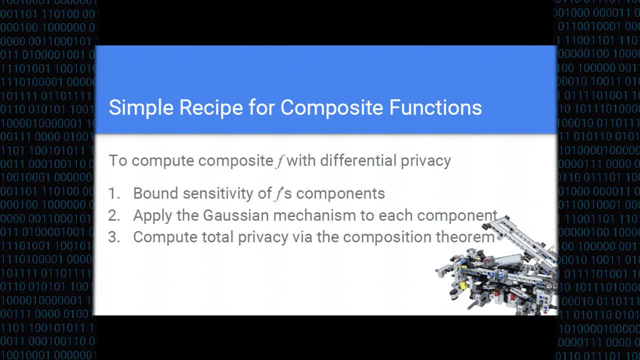 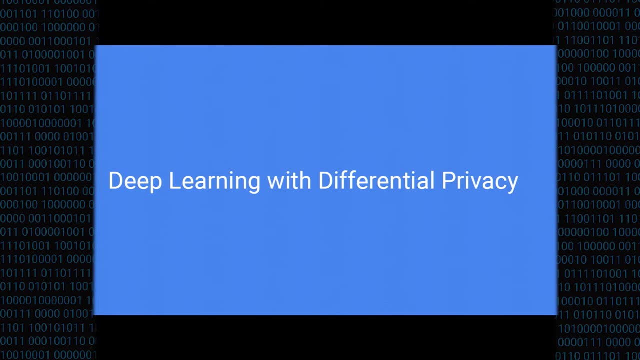 evaluating each of the components with differential privacy, for example by going through the Gaussian mechanism and then computing the total privacy loss via a composition theorem. Now I want to merge these two threads in this talk together. We want to do deep learning with differential privacy. 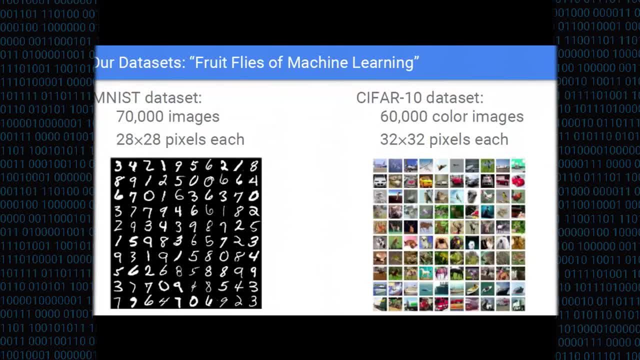 So that was our recipe for deep learning, And we'll be evaluating our algorithms on two data sets, known affectionately as fruit flies of machine learning. The first data set consists of handwritten digits- 60,000 of them. The second data set consists of 60,000 small. 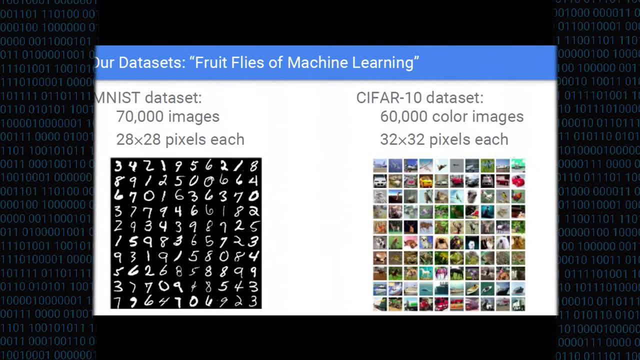 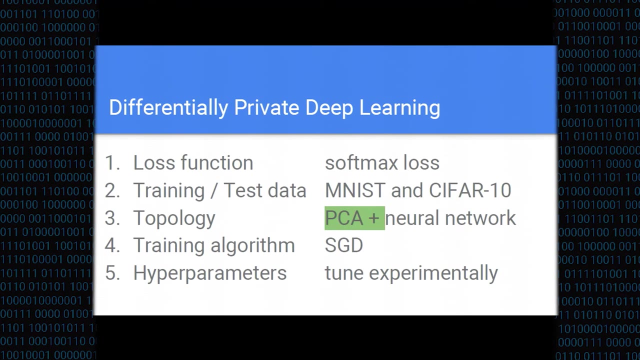 colored images drawn from 10 classes, such as cats, dogs, airplanes, ships, And in both cases, the problem that we'll be solving with machine learning models is classification task of correctly classifying these images, As the first step in adapting the existing recipe to differential. 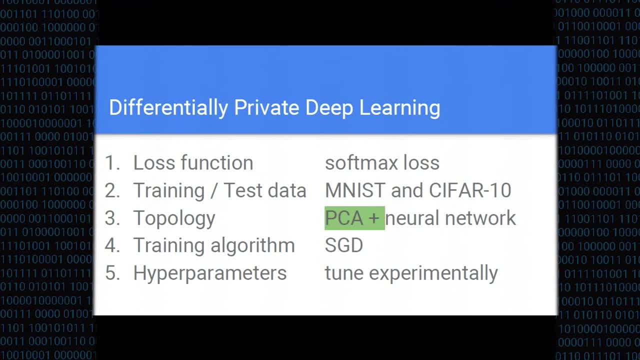 privacy. we'll end up with this, Thank you. We'll add a layer, a projective layer, that will compress the input space by projecting to the principal components. We'll be using a principal component analysis that will learn with differential privacy. 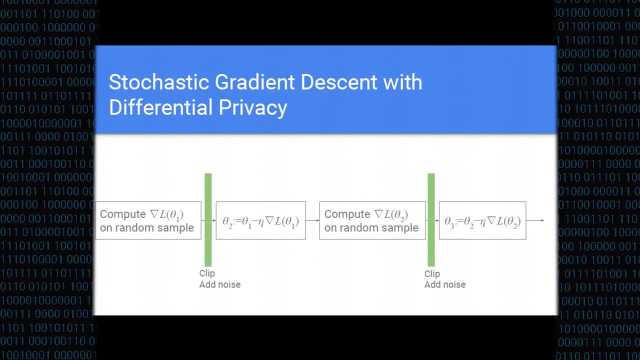 Then we want to adapt the stochastic gradient descent descent to differential privacy, And just following the recipe will be achieving differential privacy of each individual step of the stochastic gradient descent. This is not. this requires some work because by itself the gradient is not necessarily bounded. So we propose an. 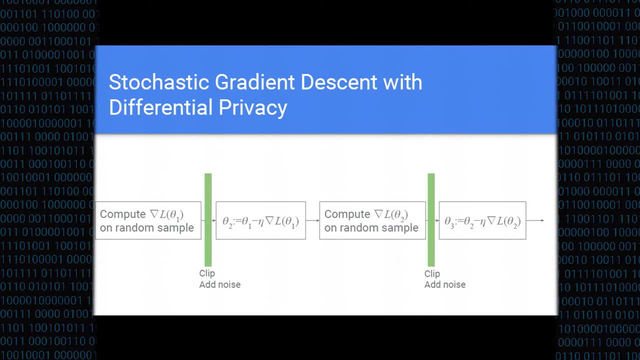 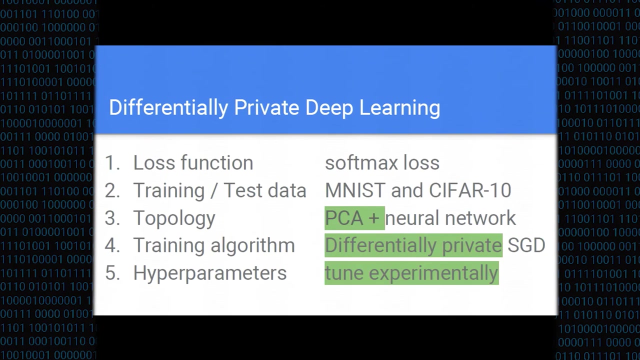 algorithm that computes the gradient together with its per-example sensitivity, And if the sensitivity is too high, it will scale down the gradient, making sure that its norm doesn't exceed a threshold, a certain threshold. Then we'll be applying the Gaussian mechanism at each step of the stochastic gradient descent. Finally, the hyperparameters. it looks like 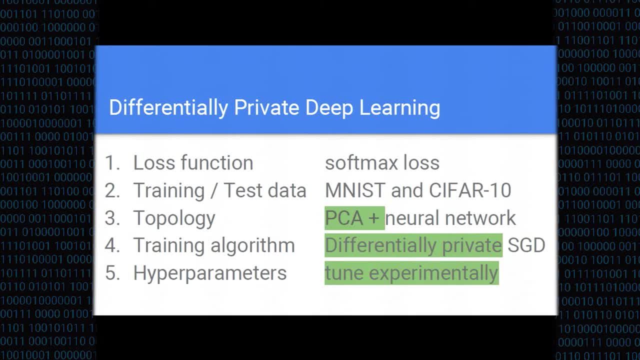 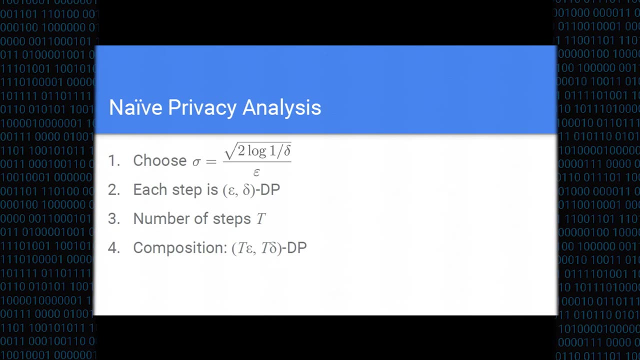 it's a little bit more complex. It's a little bit more complex. It's a little bit more complex. It's the step which is the easiest, because we only have to run our models so many times, really a few dozen times. The privacy budget that we spent on this step is really minimal. 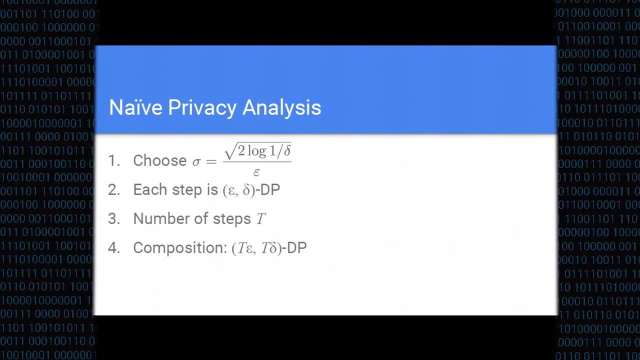 And the first time we run a system with the parameters chosen on the basis of what we are doing, what non-private systems are requiring. so the first time we ran a system until it produced a, it achieved accuracy. that was kind of decent and we computed that privacy. 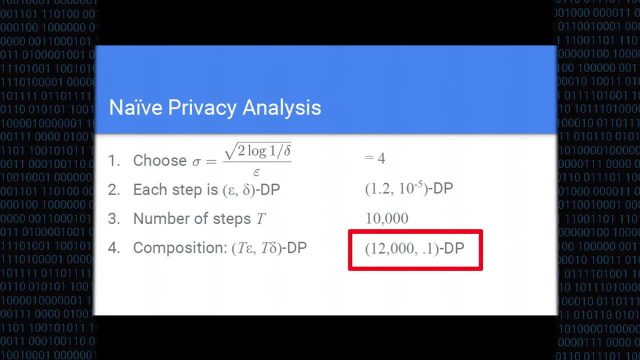 loss. we were very disappointed. So we achieved the epsilon of about 12,000, which is- and remember the address- disadvantage- is e to the epsilon. So we don't like it And we don't. So we are talking about the privacy loss or the adversarial advantage of being E to 12,000,. 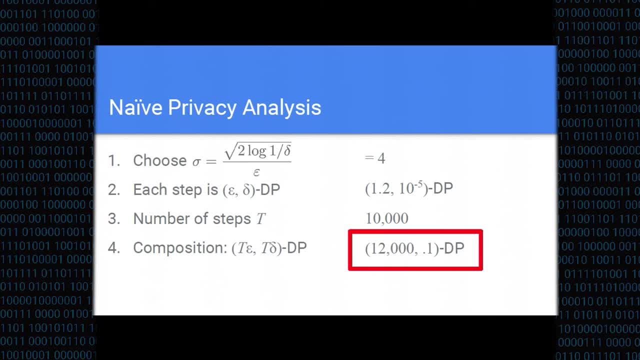 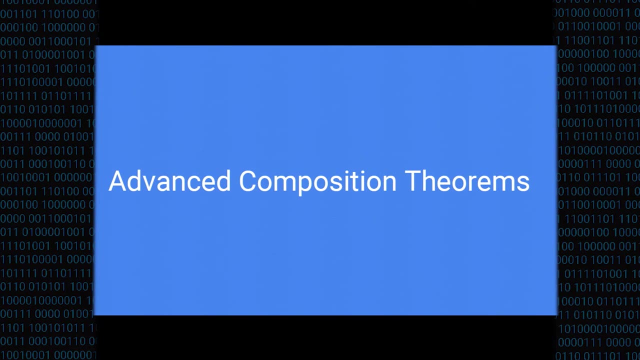 which is really a ginormous number, And it only holds with probability 90%. With probability 10% can be worse. Okay, So we need something stronger, And indeed there are advanced competition theorems that would give us much, potentially would give us much better privacy loss. 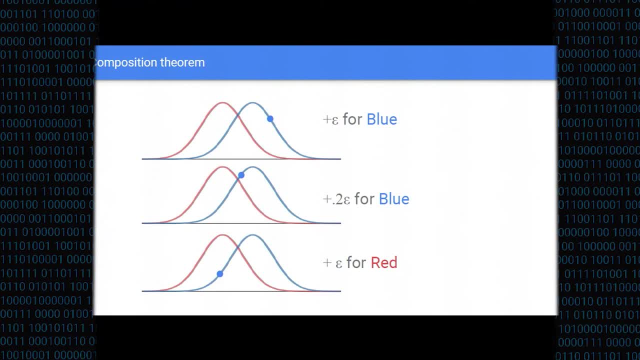 And I want to give you some intuition for why this advanced competition theorems work. So this is an example of an adversary who is trying to decide between the blue and red distribution and observes three samples from one of the distributions. So he observes the first sample from the blue distribution and it's a vote for the blue. 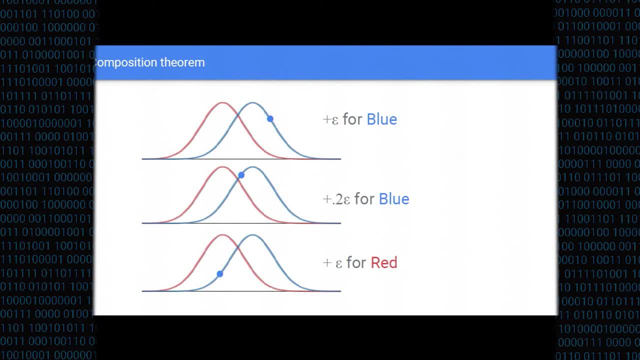 distribution. It draws a second sample from the blue distribution And it's a slightly stronger vote in favor of the blue distribution than the red It takes. it gets a sample from the blue distribution in the third case and actually it's a vote for the red distribution. 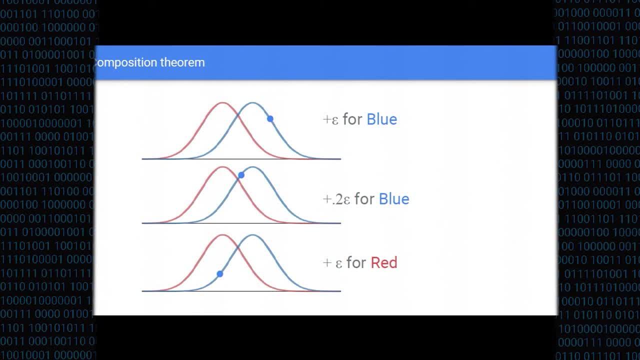 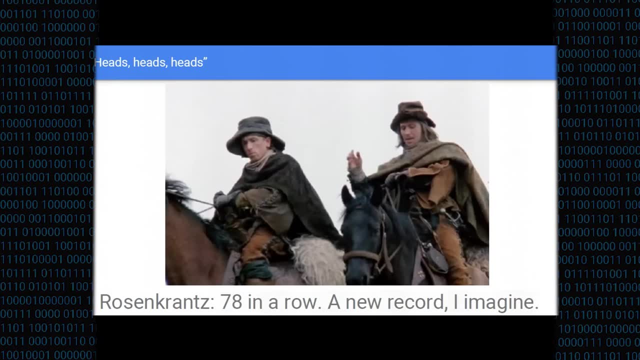 The standard. the naive competition theorem works even in the worst case, when every single of the samples is a vote in the correct direction, Which reminds me of the opening sequence of Rosencrantz and Adet, where a coin lands 78 times heads in a row. 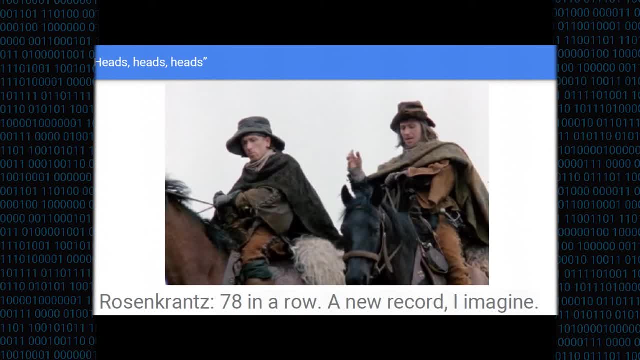 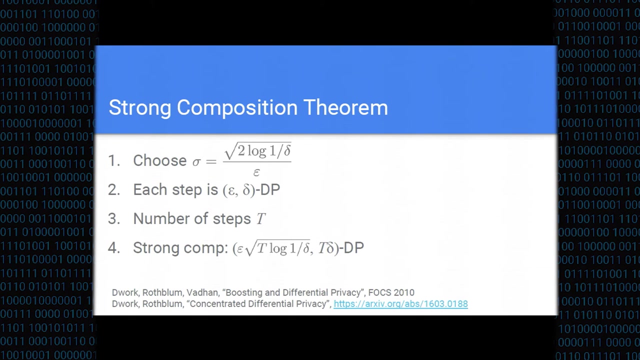 And unless we are so unlikely that it happens, we are in a much better world where the privacy loss function behaves like a random variable That can go up or can go down. The adversary can gain knowledge or be confused, So the advanced composition theorem applies. this logic models the privacy loss variable. 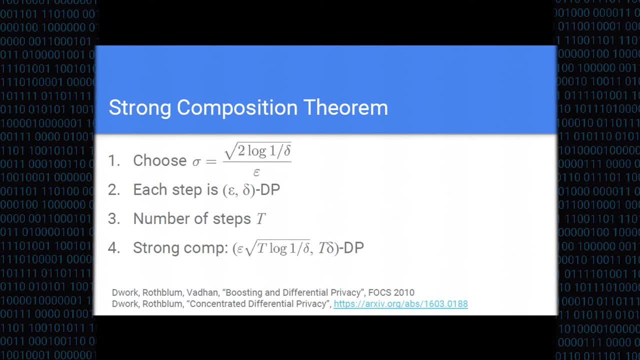 as a random variable and it roughly states that the privacy budget will accumulate in proportion to the square root of the number of steps. We apply the advanced composition theorem and we end up with a loss of epsilon of about 360, which is a big progress compared to 12,000, but still an unacceptably high number, unacceptably. 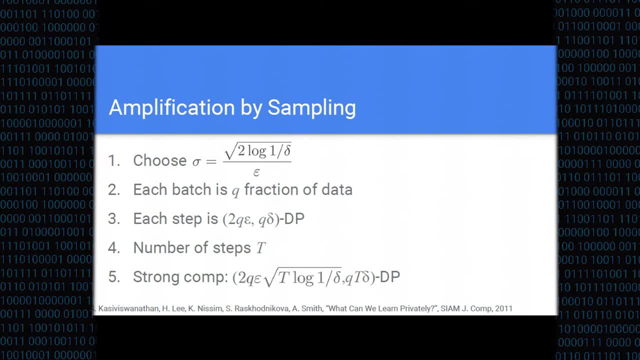 high privacy loss. We go back to the drawing board and look for ways where our analysis is loose and we observe that in each step of the stochastic gradient descent, the algorithm only touches 1% of data. We can incorporate it into our privacy analysis and once we do that, we drive down the cumulative. 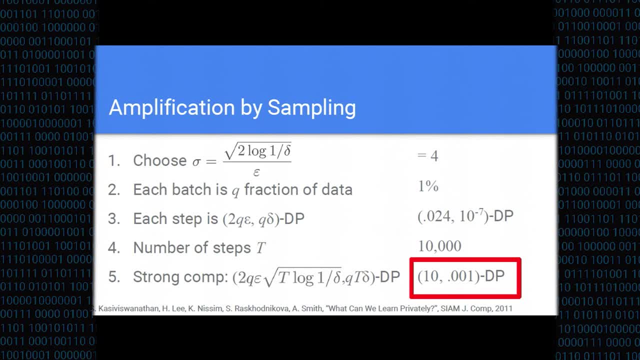 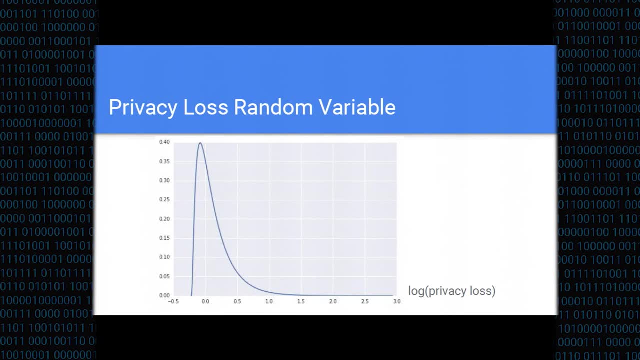 privacy loss to epsilon 10, which holds with probability 99.9%. But we want to do better And to do this, we do this. We need sharper, more accurate tools for understanding the privacy loss in the long run And I plotted here the log of the privacy loss function for the Gaussian mechanism based. 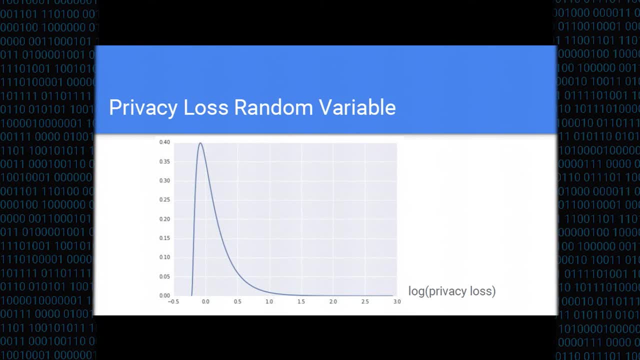 on 20% sampling And you can see from this plot that the privacy loss drops off very quickly, but it still has a long tail And in order to, In order to bound the privacy loss in the long run, we want to understand, we want to. 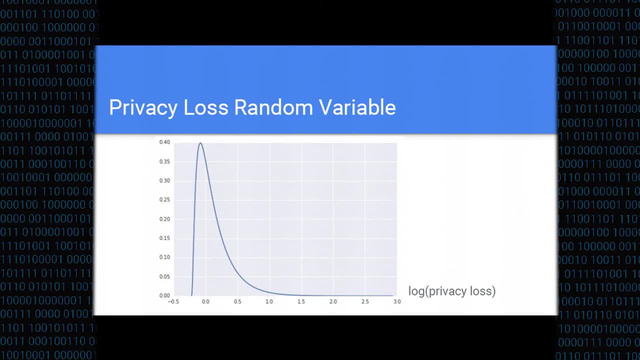 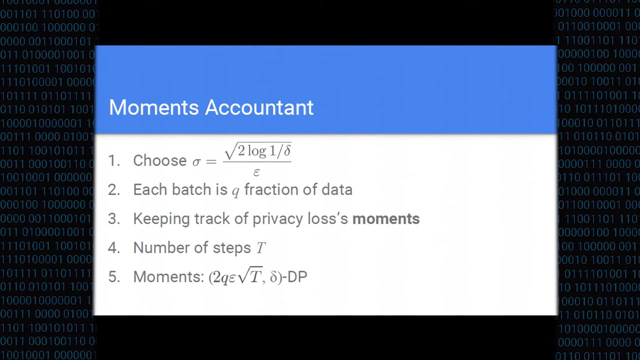 bound the. We want to have sharp bounds on the tail of this distribution And the best tools we have for doing this are the higher moments of this loss function. And in the contribution of this work that we consider important to the, To the. 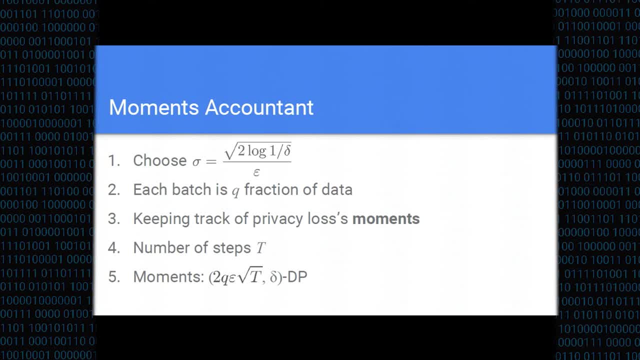 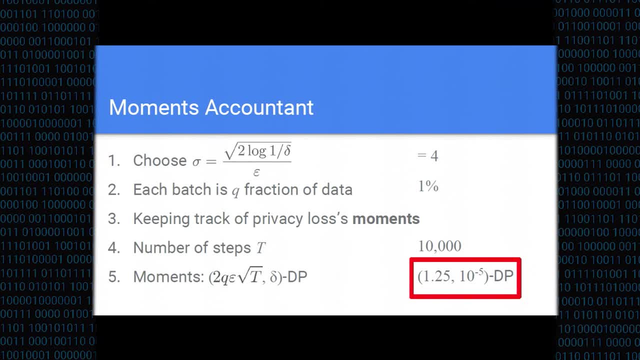 That are commonly, That are commonly That are used currently in Chrome or in Apple iOS 10.. And this privacy loss holds with probability 10 to the minus 5. And we can get the We can. If you're Want to get absence for smaller deltas, we can easily extract those from our analysis. 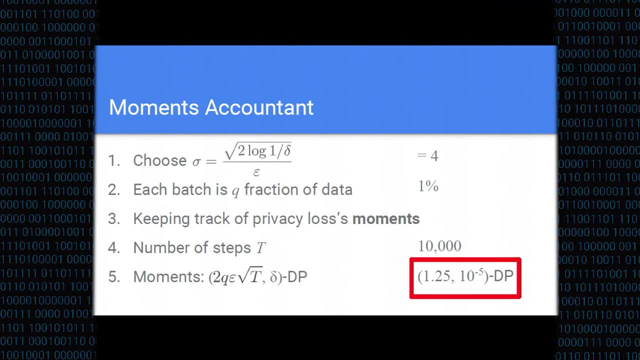 too, And here I want to stress the fact that we That we achieved- We achieved a much smaller privacy loss of the entire algorithm by going back and revisiting our analysis. We didn't change a single step in our original algorithm. We kept redoing the analysis by bringing insights from probability and algorithm. 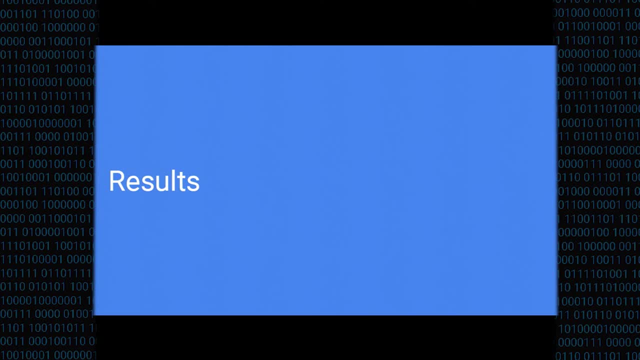 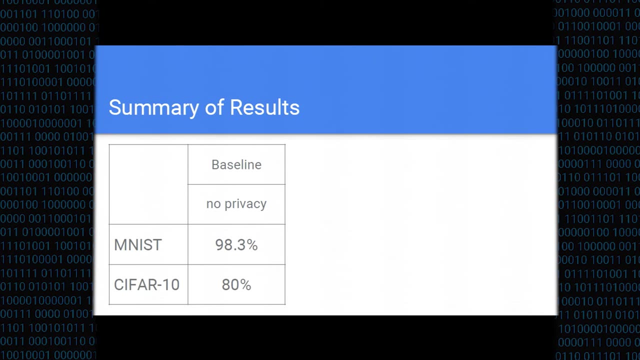 And algorithms. So, So, So let me bring up the results of our work. So this is the baseline that we are comparing ourselves with, Where, on MNIST, the baseline models achieved accuracy of 98.3%, with no privacy. 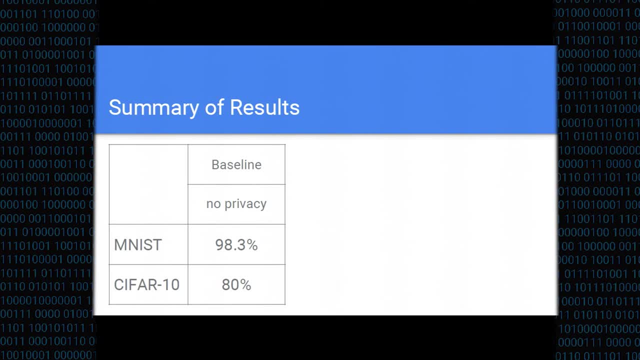 On the CIFAR-10, the colored images. we've got 80% accuracy. In the prior work from CCS last year, which achieved accuracy on MNIST of 98%, this prior work reported absence per parameter of the model And there are tens of thousands or even hundreds of thousands of these parameters. 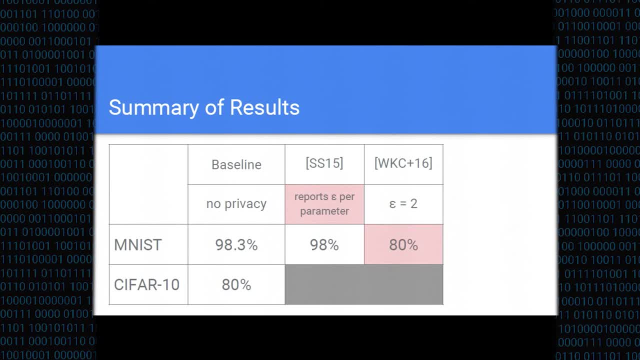 So the total cumulative privacy loss was about 2,000.. And again we are talking about e to the epsilon, in the, The actual adversarial advantage, And in the concurrent work by Wu et al they achieved a much more decent epsilon of 2.. 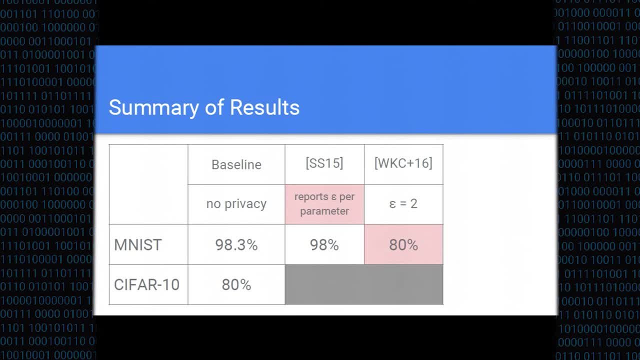 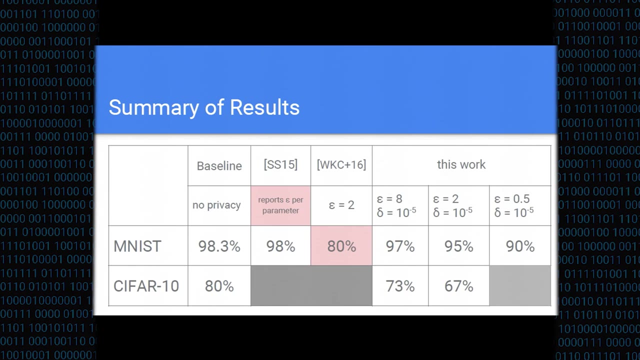 But by training a convex model, which is a much more narrow class of models, and their accuracy on MNIST was 80%, a long way off of the existing, prior Of the existing state of the art. So, Finally, For our results, we achieved 97% accuracy on MNIST, with epsilon of 8.. 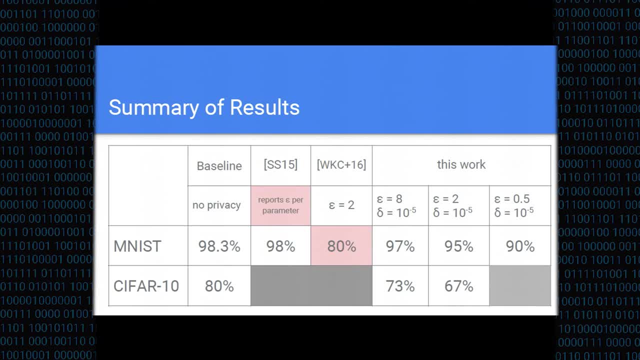 And it increases slightly as we turn off the privacy parameters On CIFAR. the gap between the baseline and our privacy-preserving mechanisms is larger And I invite you to try to improve on our answers, On our results And, To conclude, 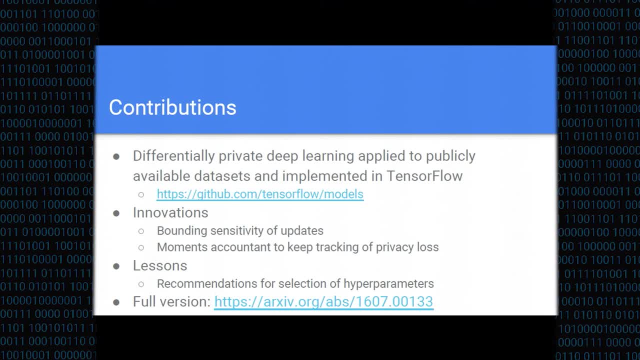 We demonstrated that differential private deep learning can be Can achieve reasonable accuracy numbers. We ran our analysis on publicly available data sets, Encouraging, Basically bringing competitiveness, And And We implemented our work in TensorFlow and open-sourced our code. 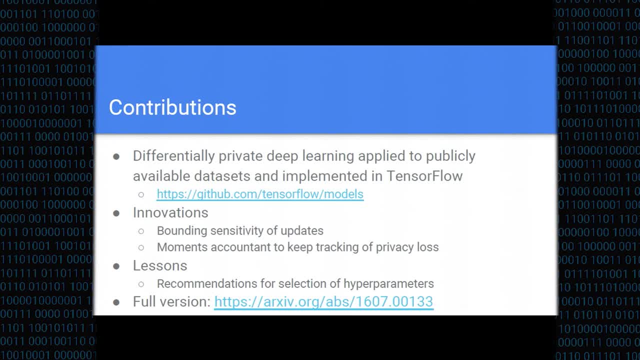 It required. There were several algorithmic advances in our work And there are all shared in paper and code. There are lessons, if you want to do similar work, that are in the full version of the paper that is available on archive. Thank you. 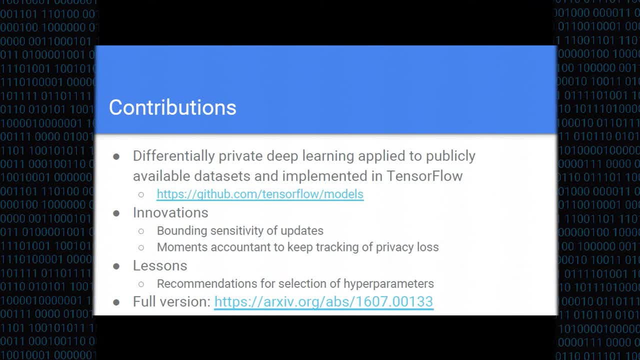 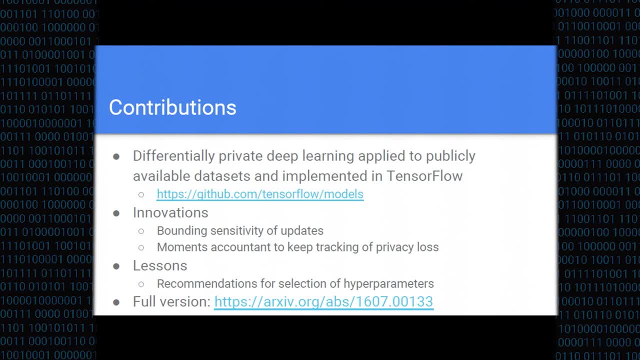 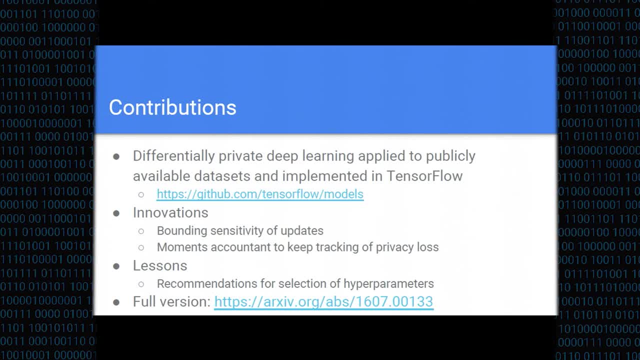 in noise salvation part, Yeah, So. So this is a very simple type. So This is a very simple question. because the Gaussian distribution is more concentrated, So it gives somewhat weaker privacy guarantees, because Gaussian distribution doesn't achieve pure differential privacy but because it tails drop off more quickly. 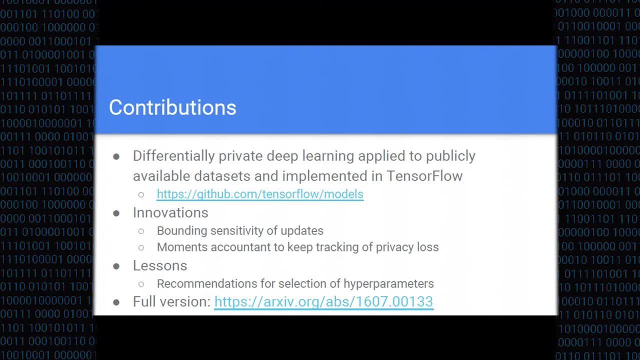 then it ends up having a much smaller variance. But intuitively it's usually the exponential mechanism can get the best utility performance, so that's Okay. so for the exponential mechanism: strictly speaking, any mechanism can be cast as an exponential. so by saying that, 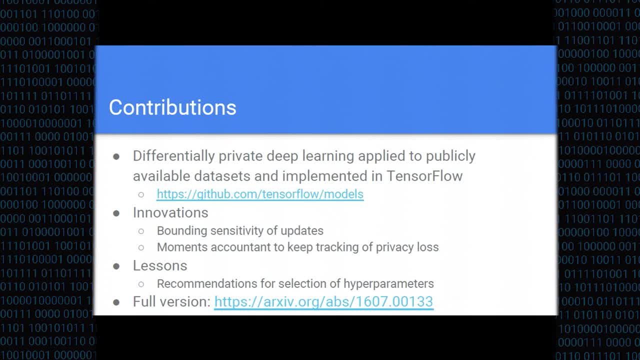 you can cast any differential private mechanism as an exponential mechanism. So exponential mechanism doesn't really narrow the space of mechanisms. Okay, thank you. More questions, Hi, this is from Penn State University. Yeah, I have two questions actually. The first question is: I realize you use PCA in front of a neural network. 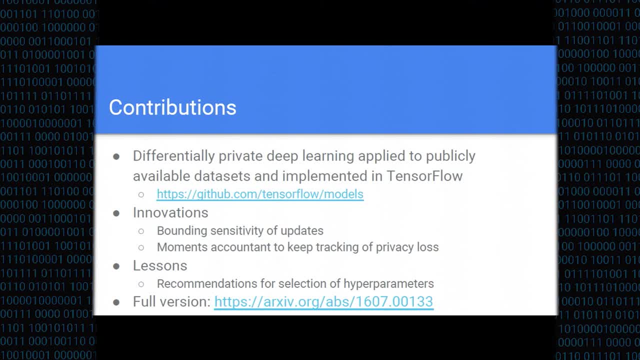 That's correct, And one of the big advantages for a deep neural network is deal with high dimensional data. Yes, Another reason: it gives us better performance For PCA. when you do the dimension reduction, apparently you will see the performance drop. 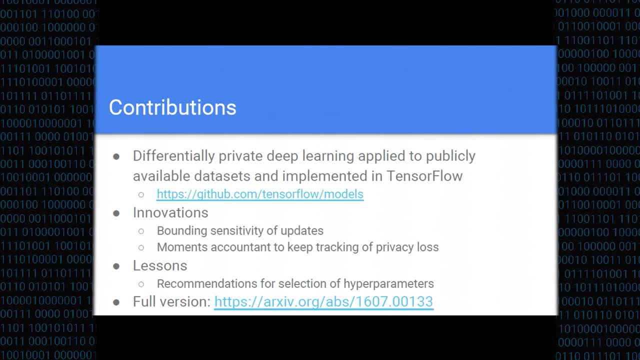 out significantly. That is also shown in your slides. So my question is how practical this, This solution, could be in the real world. That's my first question. So I don't think that the drop off compared to the baseline can be attributed to. 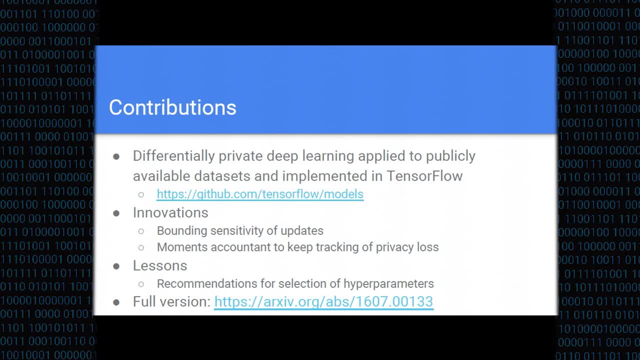 Is mostly due to the PCA step. I don't think it's true. The PCA is actually, at least on the MNIST. CFR data sets- doesn't lead to big drop in performance. Okay, And the PCA it's. I think it compresses the input images by a factor of 10.. 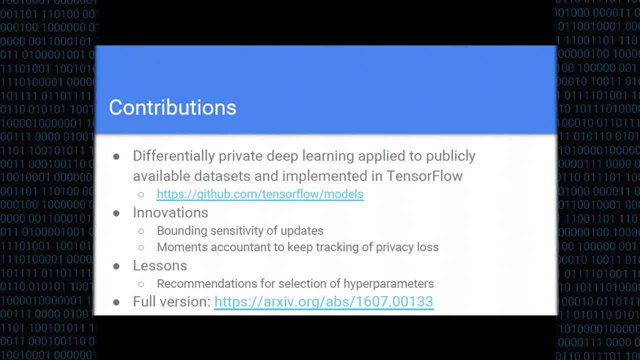 But it's a projection to the principal components. So really kind of the information is mostly preserved by the PCA step, So I wouldn't rule it out completely. Yeah, My understanding is like when you deal with the MNIST data set, it's definitely include. 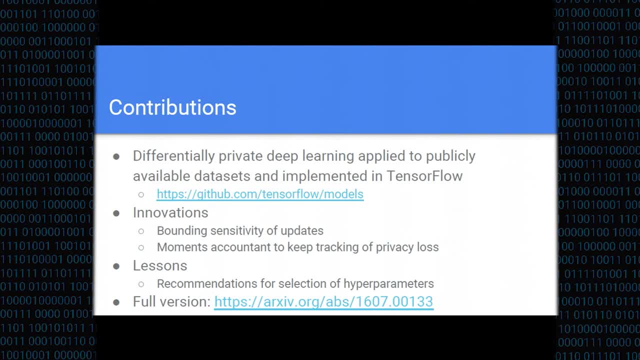 Because it's white and black, it's definitely include a lot of non. Yeah, Yeah, Yeah Yeah, It's not quite useful data, So that's the reason we'll do the dimension reduction. Yes, You still see the performance maintained in a high accuracy. 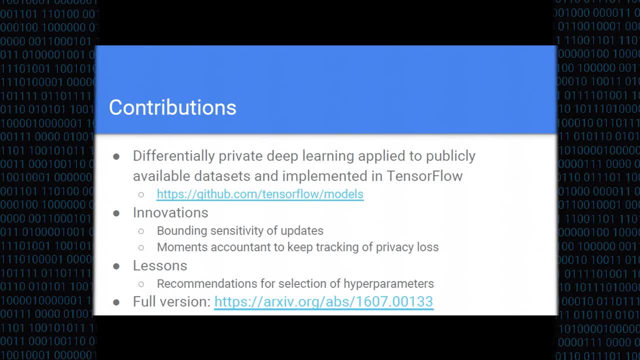 But actually when you deal with the CFR 10, maybe CFR 100, I don't know whether you did that or not. So that includes a lot of colorful information. We'll do the dimension reduction. It definitely lose a lot of useful information. 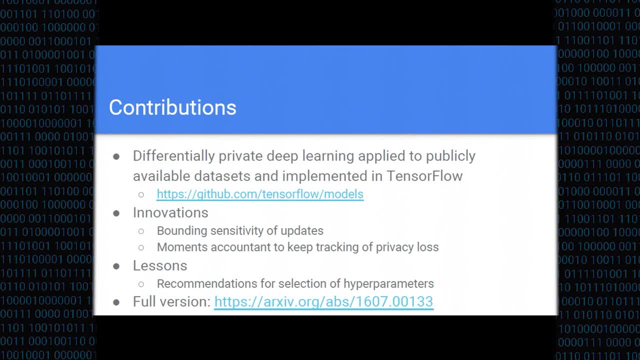 That is my personal understanding. Okay, That's the first statement. Yeah, The second question that I have is how possible this approach could apply. So, for example, if you have a deep neural network architecture like R and N recurrent neural network, 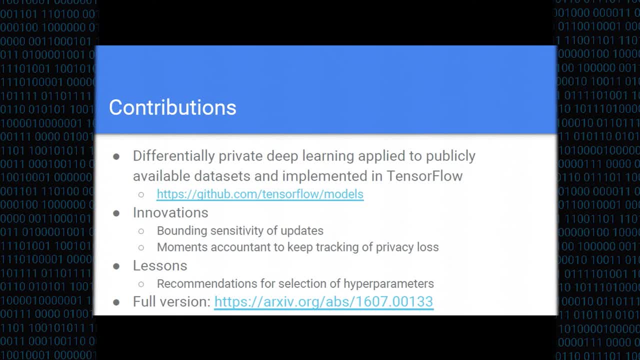 Okay, So our hope was to. So that's an excellent question and something that is on our plates, But we hope that this work is general enough and its lessons are transferable enough to other types of neural networks. So, in particular, the stochastic gradient, descent. it's. 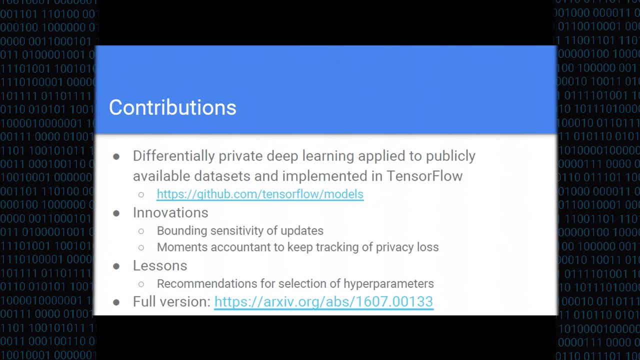 What we do can be generalized to all other methods that are based on gradients. So I would say that it's definitely It might work, Or it might require some new ideas to make it truly practical. Okay, Thank you. We have time for one more question. 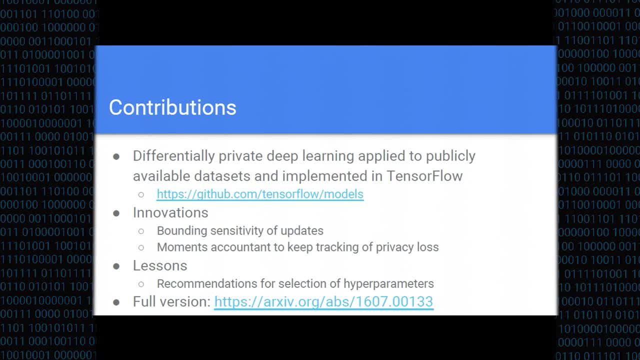 Hi. Thank you for the talk. I wonder if you run model inversion on the networks and if you have an intuition of how the results look like. Can you say again If you run the model inversion attacks by? I see Fredrickson et al. 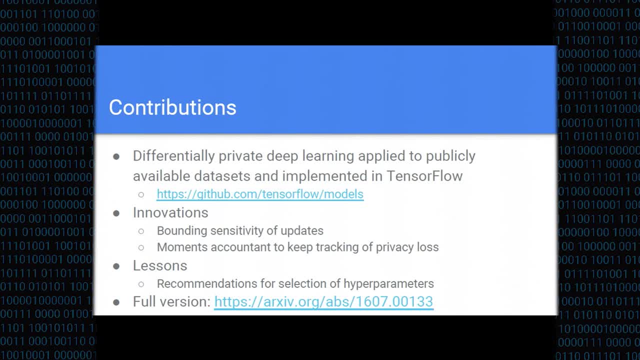 Yeah, Yep, yep. So we haven't done, We haven't run the attacks themselves. As Fredrickson et al say, differential privacy is a defense against their attack, So there are definitely theoretical bounds that you can derive that show that their attack.